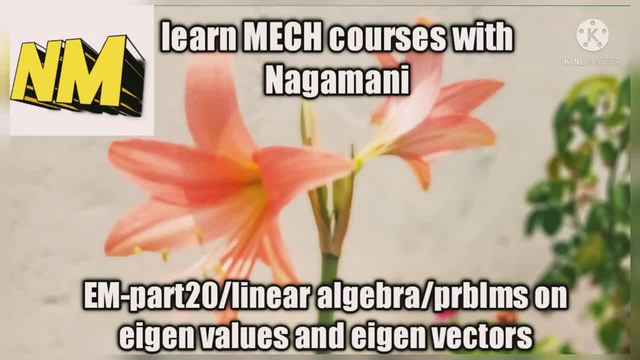 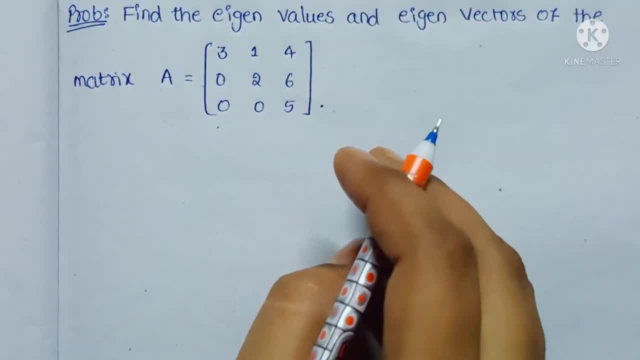 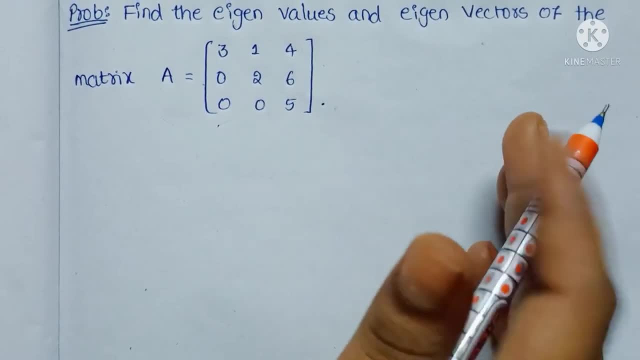 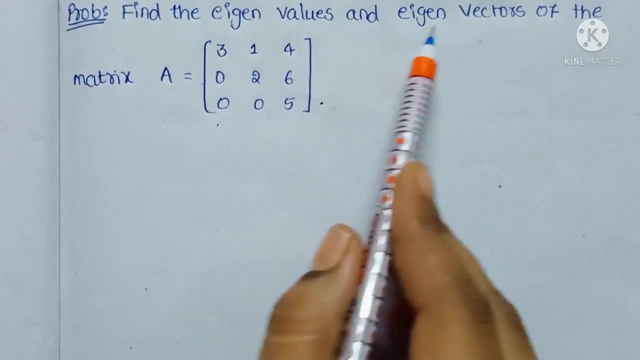 Hi friends, welcome to my channel, NM learn, make courses with Nagamani, And today we will see how to find the characteristic equation and eigenvalue sign, eigenvectors. So don't skip the class and watch till the end. Now, coming to the problem, They are given a matrix and they are asking to find the eigenvalue sign, eigenvectors. If you see the solution, 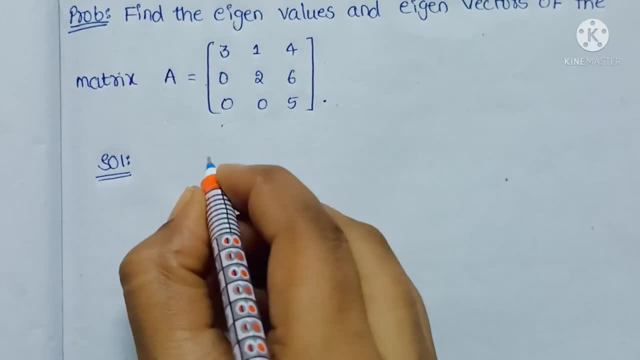 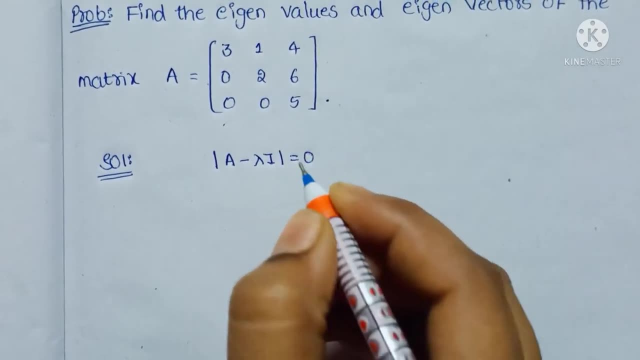 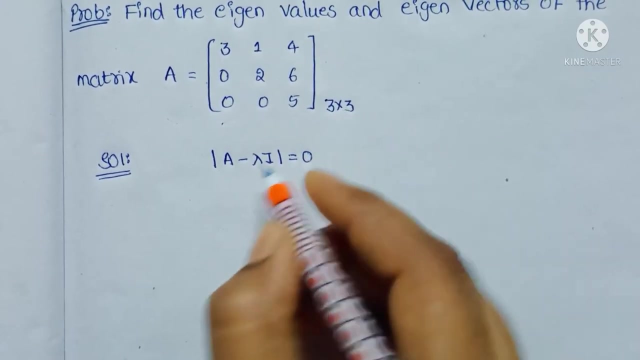 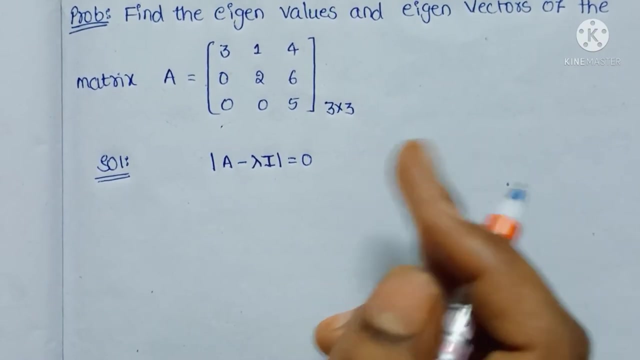 And we know how to write the characteristic equation where modulus of A minus lambda I, which is equal to zero. Okay, here, a matrix is these three by three matrix. they are given and lambda is a scalar quantity, where I is identity matrix. that is one zero, zero, zero one, zero, zero, zero one. Now I'm writing here: Okay, three by three. 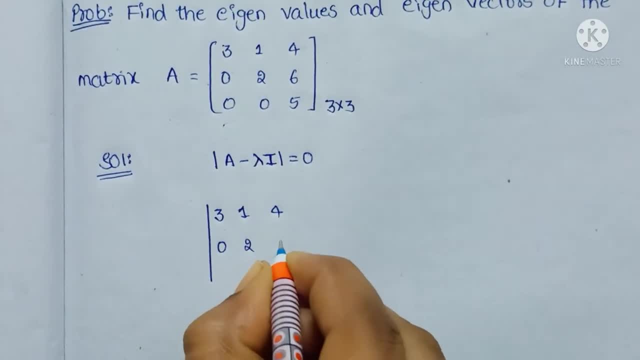 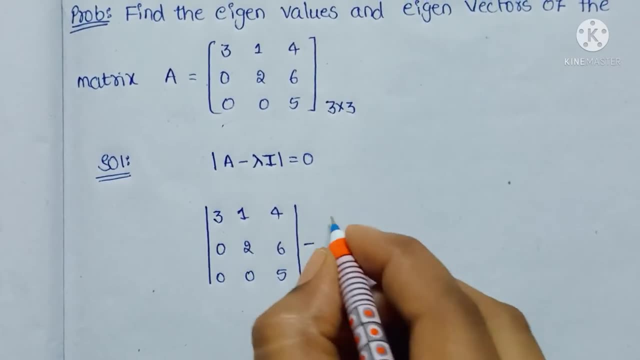 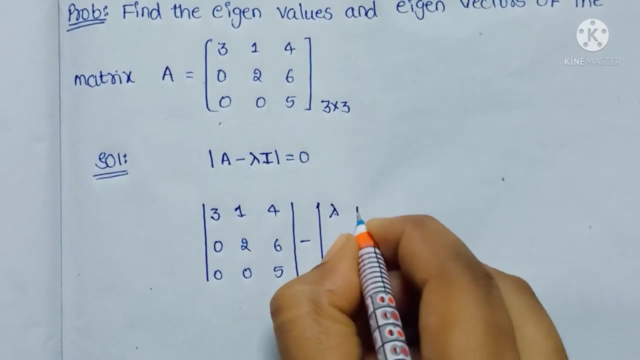 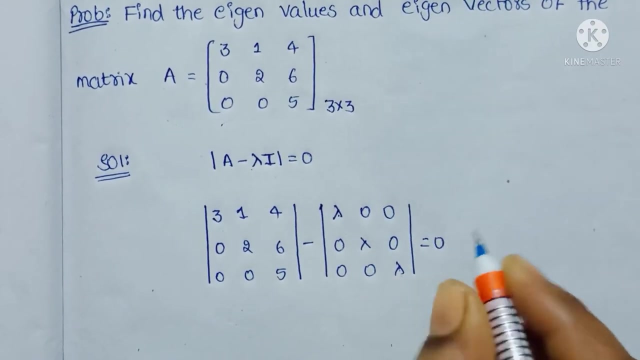 One four zero two, six zero zero, five. This is the matrix minus lambda. into I am writing directly where one zero, zero. So I'm multiplying with lambda, lambda, zero, zero, zero, lambda, zero, zero, zero, lambda, which is equal to zero, And subtracting a from lambda I matrix. 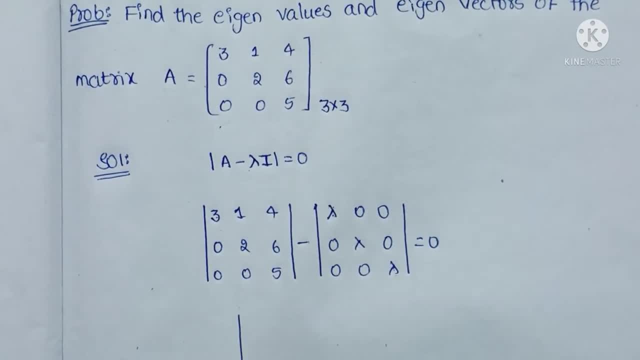 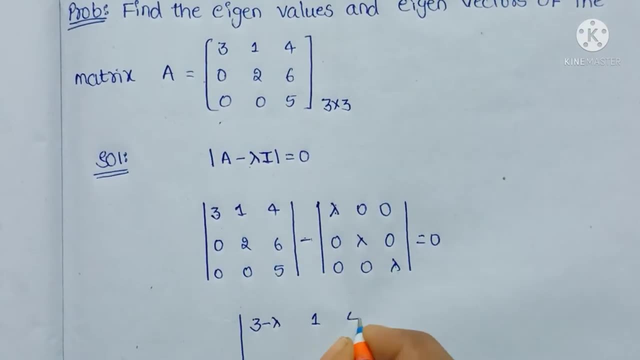 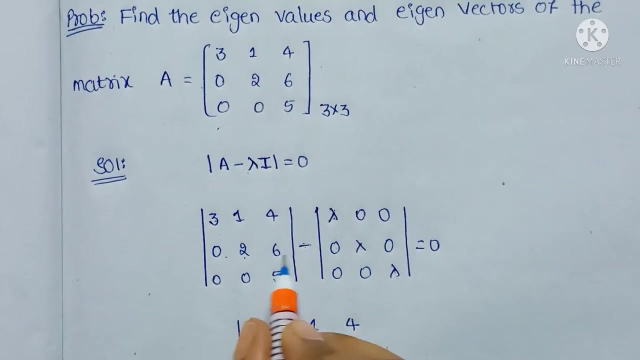 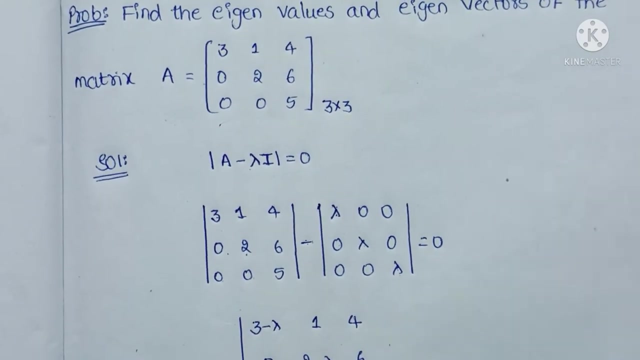 Then we get three minus lambda here three minus lambda and one minus zero. one. four minus zero, four here zero minus zero, zero and two minus lambda here and zero. six minus zero, six zero minus zero, zero and zero minus zero, zero. here five minus lambda. Okay. 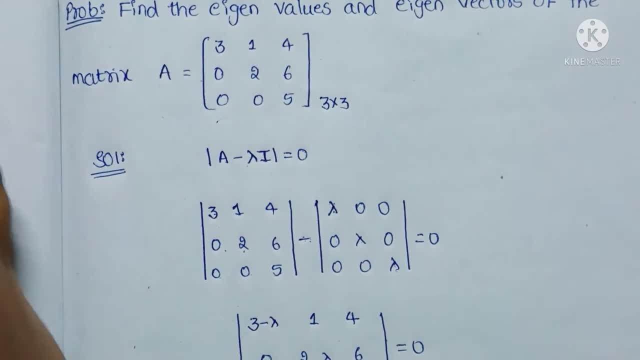 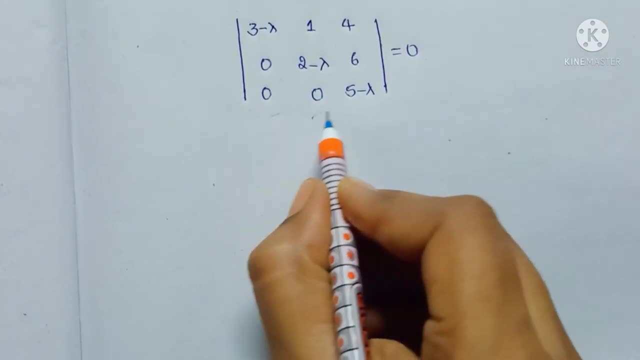 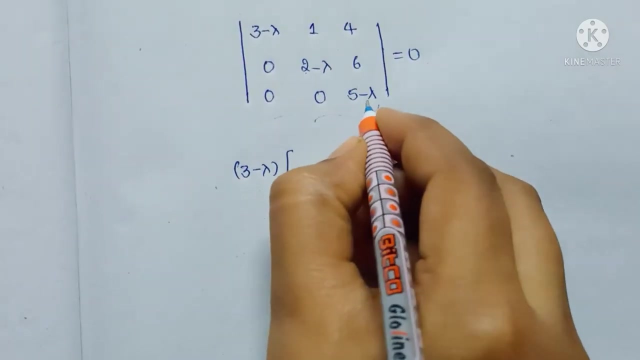 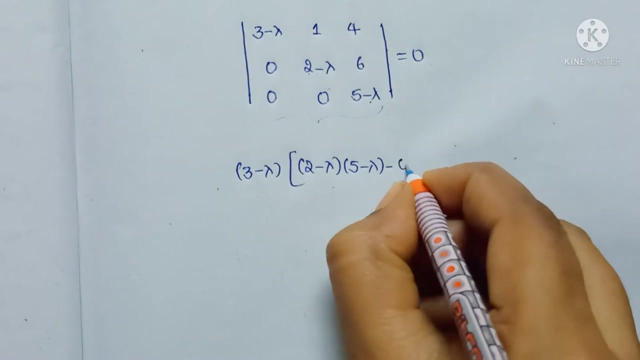 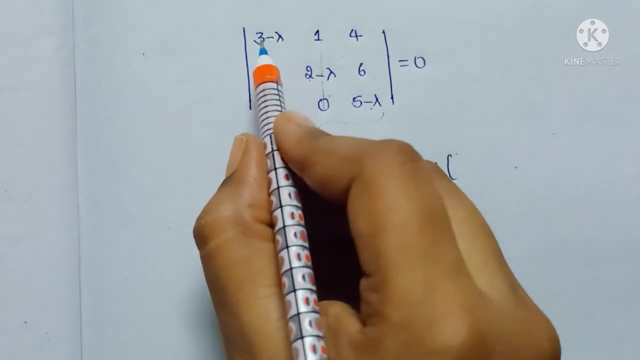 Now we are finding the determinant of this matrix. Now we are finding the determinant of this matrix. Okay, Here, three minus lambda into two minus lambda into five minus lambda. Okay, Minus zero into six. zero minus here, one into. If you close this row and this column, then zero into something. zero minus zero into six zero. 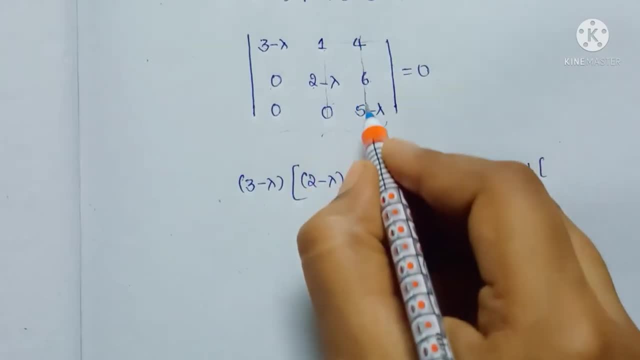 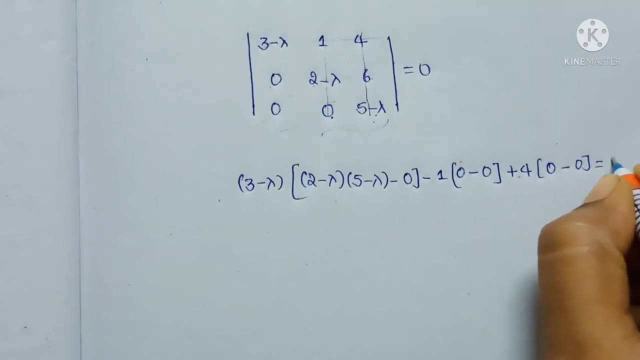 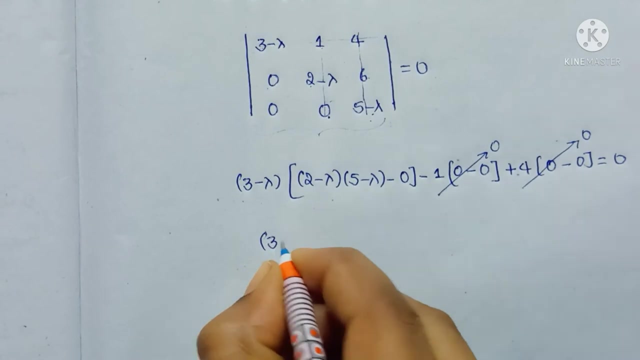 Plus four into here. if you close this column and this row, we are getting zero into zero, zero minus zero into something zero which is equal to zero. directly here we get zero and this is also zero. If you see here, three minus lambda into two minus lambda into. 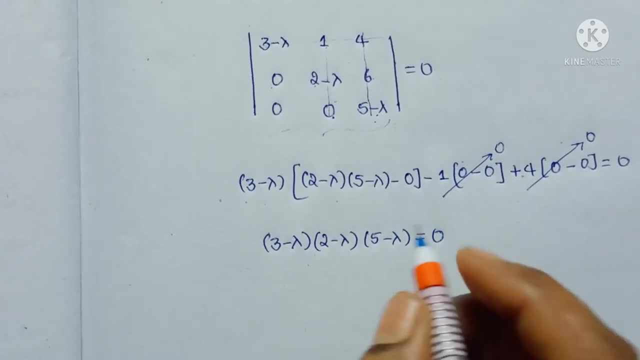 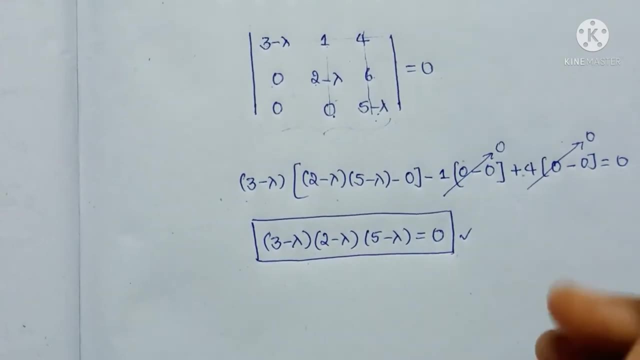 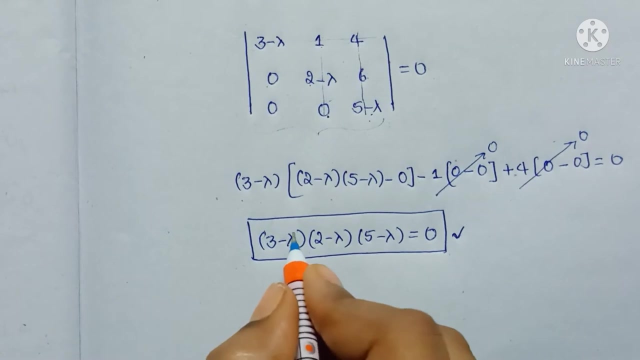 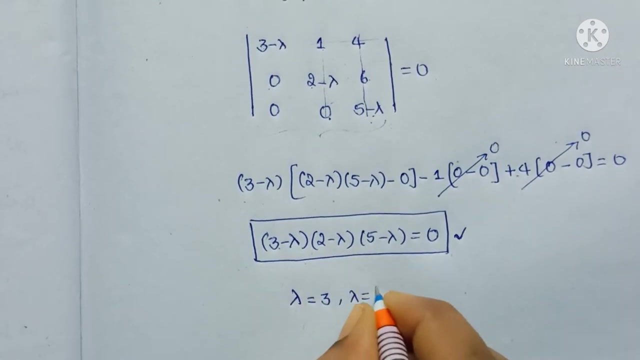 If you see here, three minus lambda into two minus lambda, into five minus lambda, which is equal to zero, by expanding these equation we get characteristic equation. now I'm not expanding, so by expanding this we get characteristic equation. from this we are finding eigenvalues that are lambda values here: lambda equal to three and lambda equal to two, lambda equal to five. 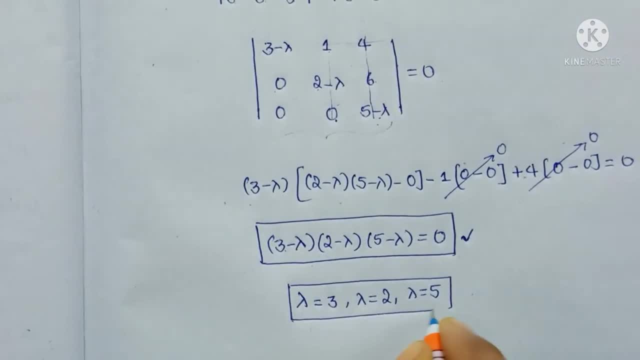 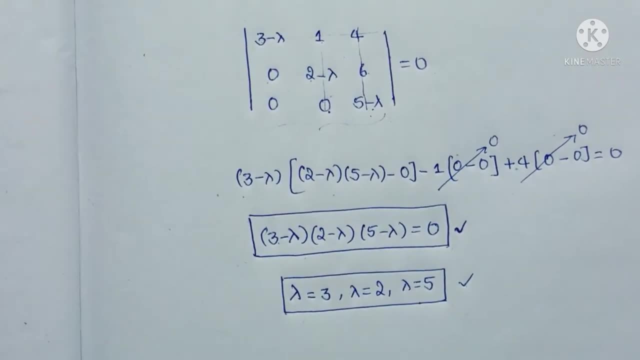 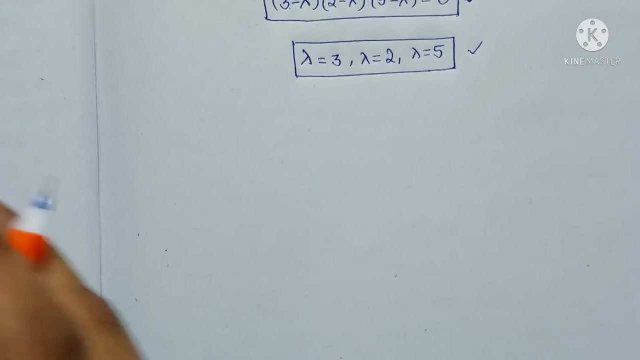 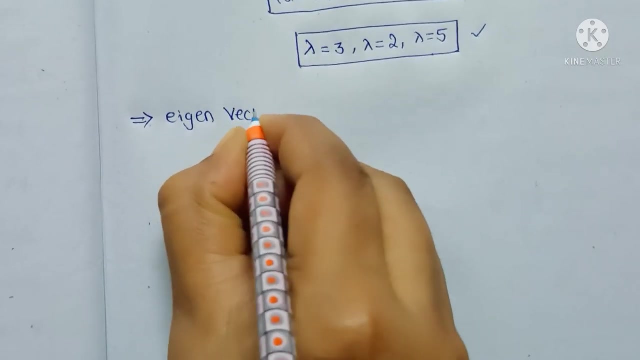 Okay, These are the eigenvalues of Given matrix. okay, these are the eigenvalues for given matrix. and now coming to the eigenvectors: how to? by using these eigenvalues, we are finding eigenvectors. okay here, if you see, eigenvectors for lambda equal to two is okay. 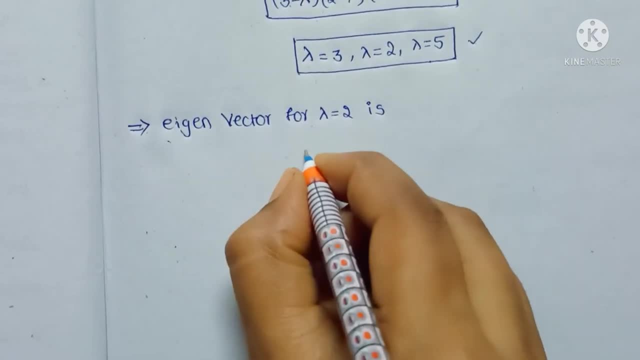 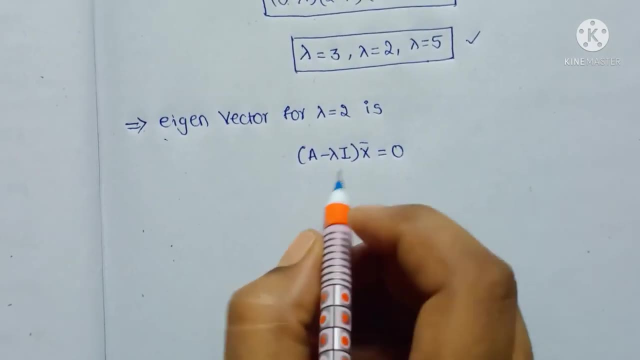 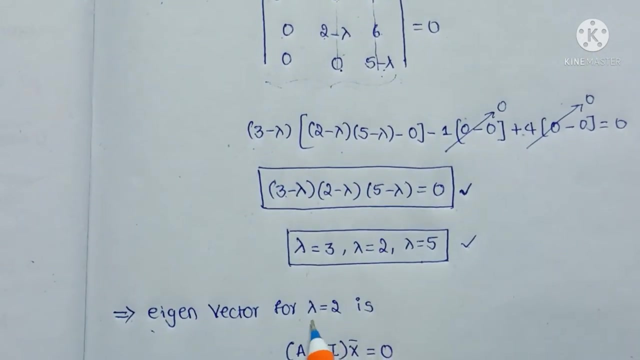 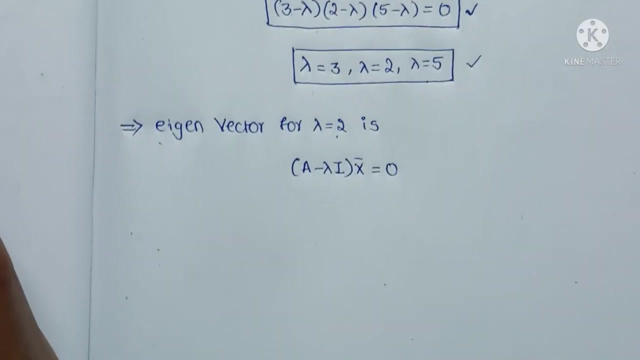 Here we are finding The eigenvector, for we are using only one equation: a minus lambda i into x bar, which is equal to zero. here we know a minus lambda i matrix and directly substitute lambda equal to two in this matrix. okay, By Sorry, I'm writing here. 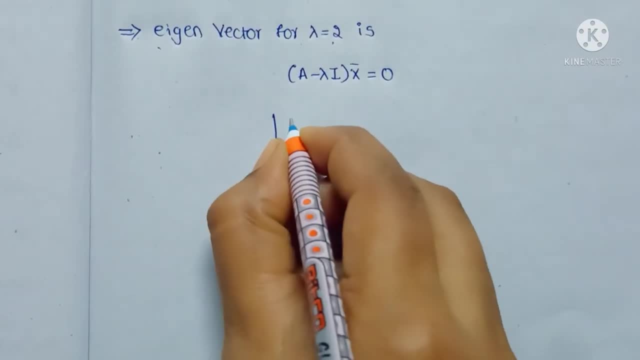 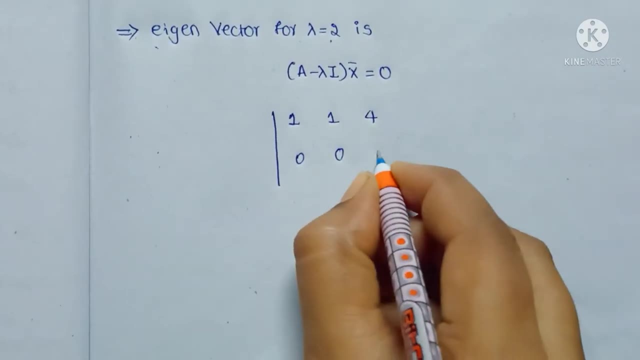 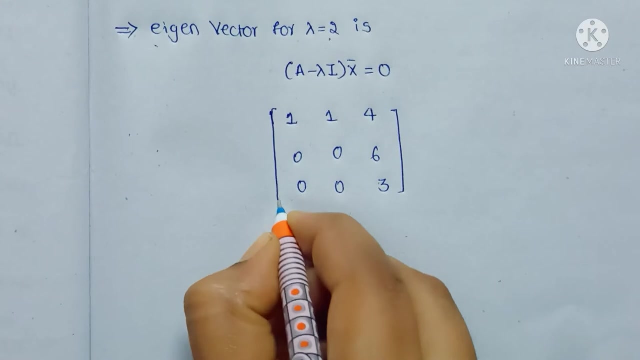 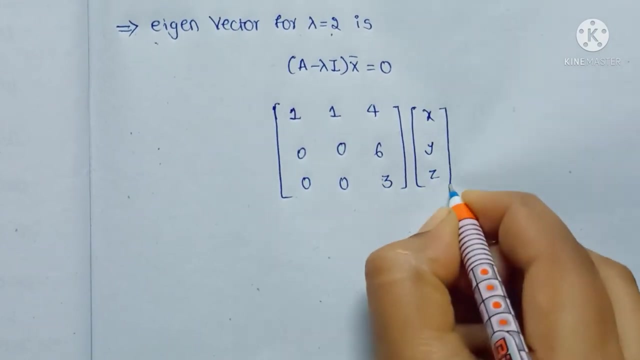 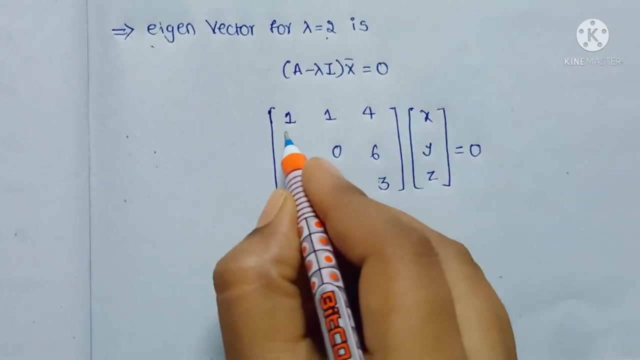 Directly Okay. Three minus two, we get one. There is no change in one and four zero two minus two. zero six. zero, zero. five minus two, we get three. okay, This is the a minus two i matrix, and here x bar is the x, y, z vector, which is equal to zero. and this matrix we are writing in equation form. if you multiply with this row into this column, we get: 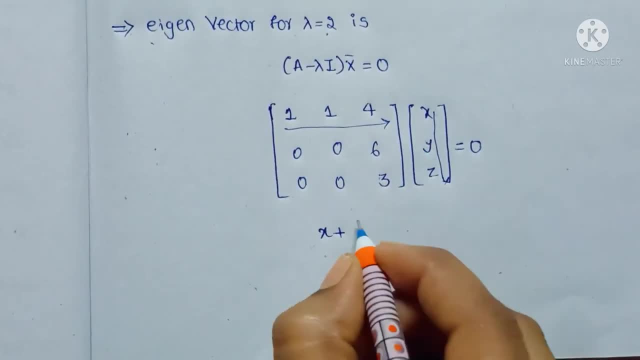 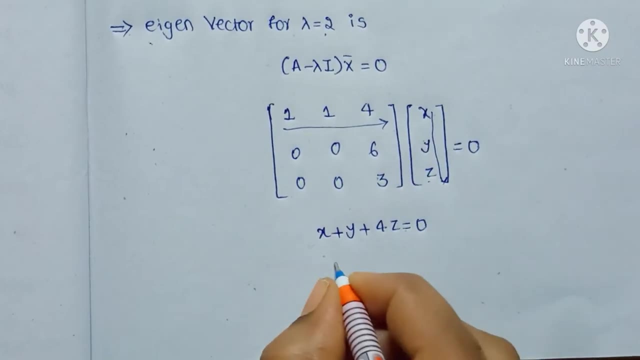 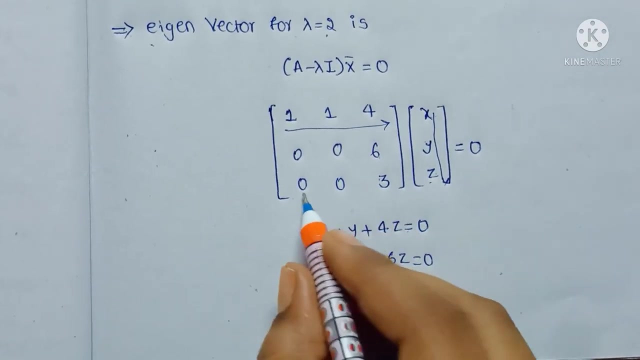 Finally, one of x a x plus one into y, y less four into z, Four, z, which is equal to zero. and zero into x, zero plus zero into y, Zero plus x into z, six, z, which is equal to zero. similarly, here also zero into z, zero, zero z into y, zero plus three into z, three, z, which is equal to. 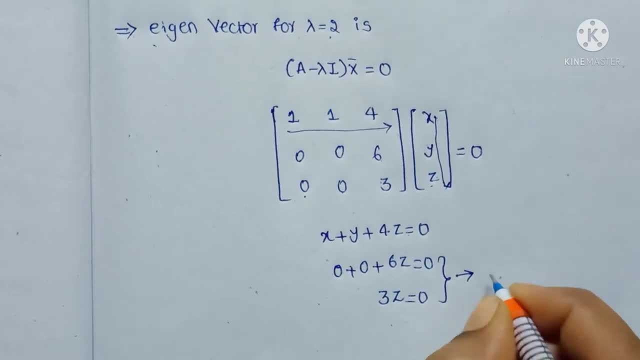 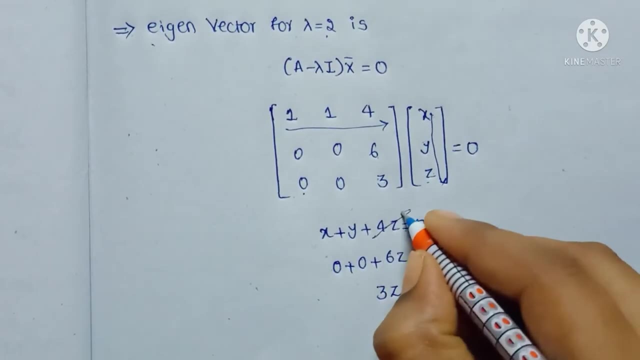 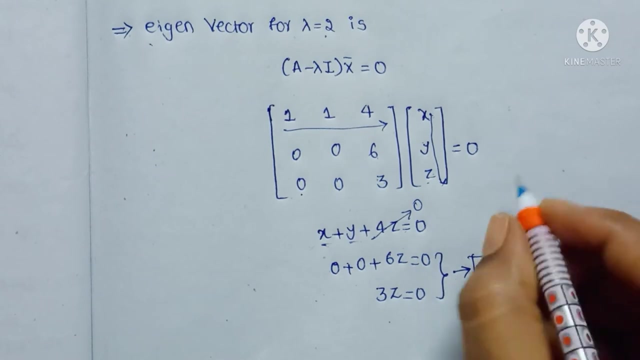 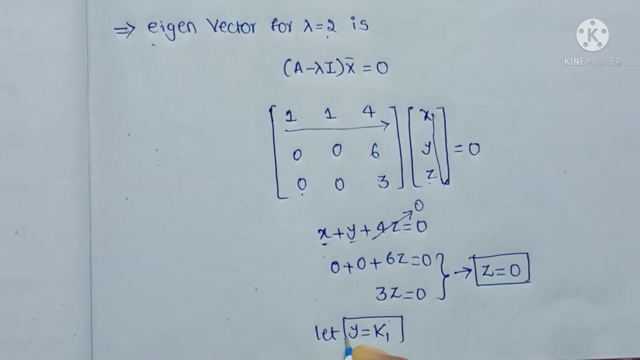 Zero. from these two equation we can conclude: Z is Equal to 2. okay, z is equal to 2. here 4z, which is equal to 0. in order to find x and y, we have to know any one value. so we are assuming let y equal to k1 parameter. okay, we are assuming y equal to. 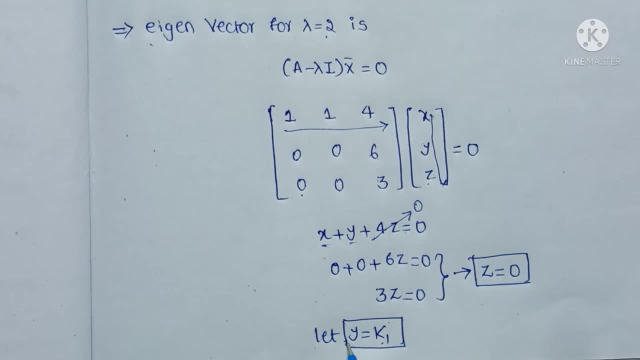 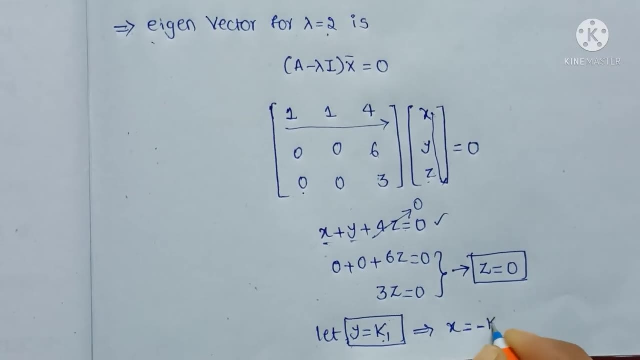 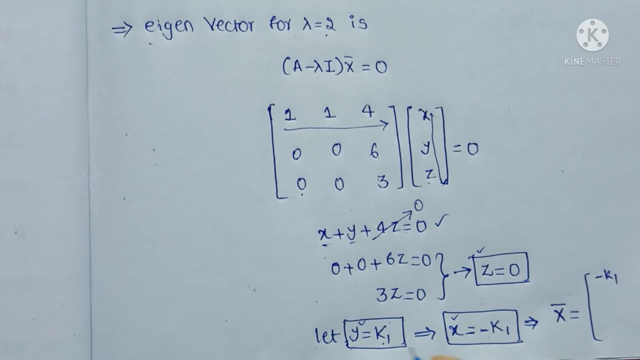 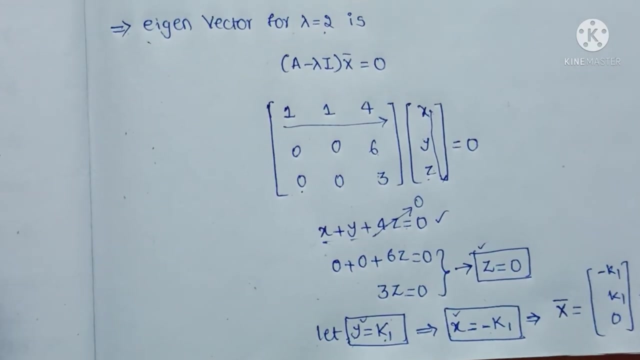 k1 parameter by substituting, by substituting y equal to k1 in this equation we can find x equal to minus k1. so now we know x, y, z values. now we are writing matrix. vector form is x, bar is equal to here: x is minus k1, y is k1 and z is 0. okay, and if k1 by common, k1 as common. 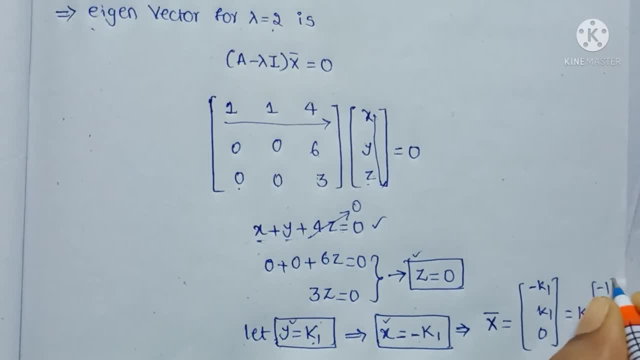 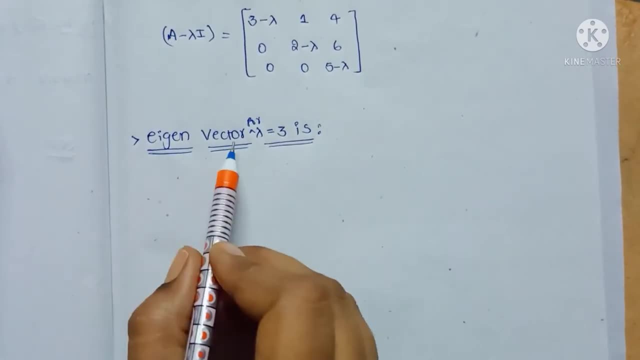 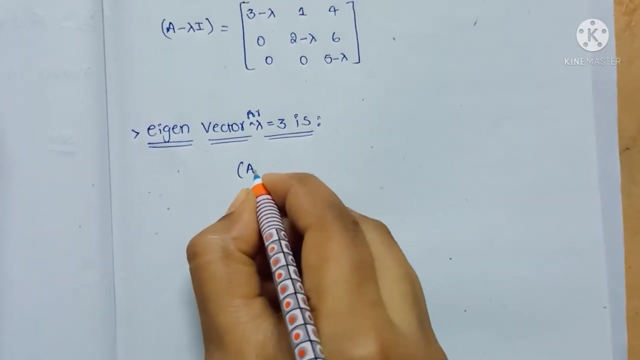 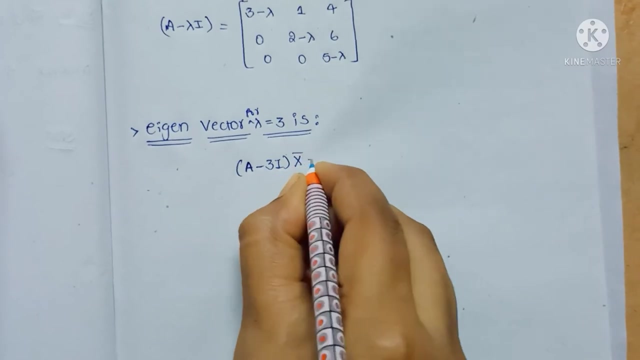 then we get minus 1, 1, 0. i wrote the a minus lambda i matrix here. okay, now we are finding eigenvector for lambda equal to 3. okay, if you see the characteristic, sorry, if you see the vector matrix is a minus lambda is 3 into i, into x bar, which is equal to 0. so substitute to lambda equal. 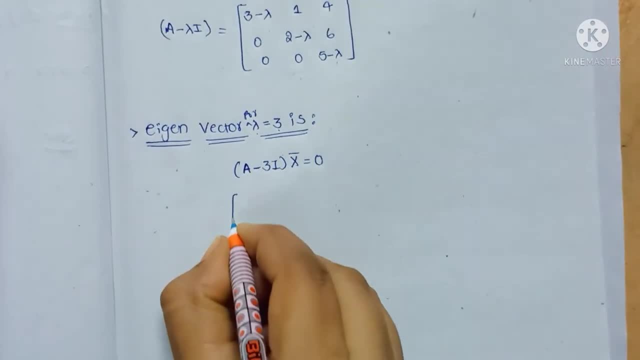 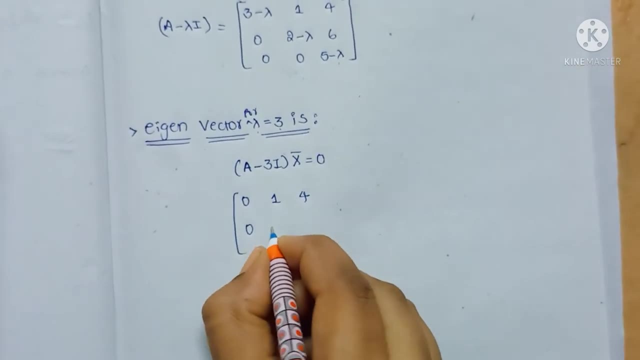 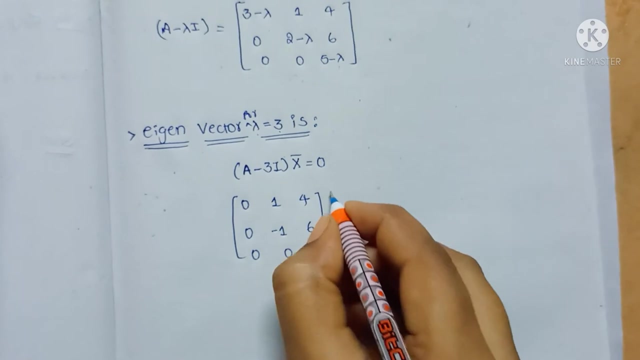 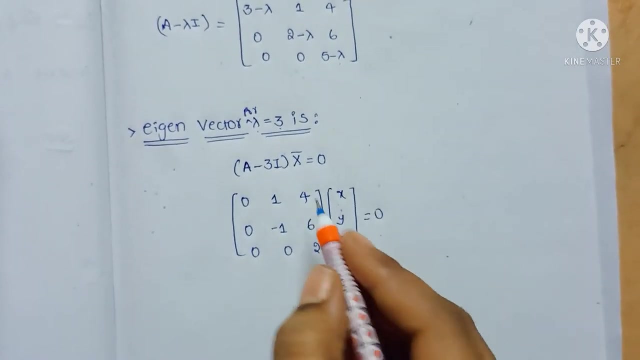 to 3 in this matrix. matrix, okay, we will get 3 minus 3, 0 here 1, 4 0. 2 minus 3, we get minus 1. here 6, 0, 0. 5 minus 3, we get 2. and where x bar is the vector form of x, y, z, which is equal to 0. and this matrix we are writing. 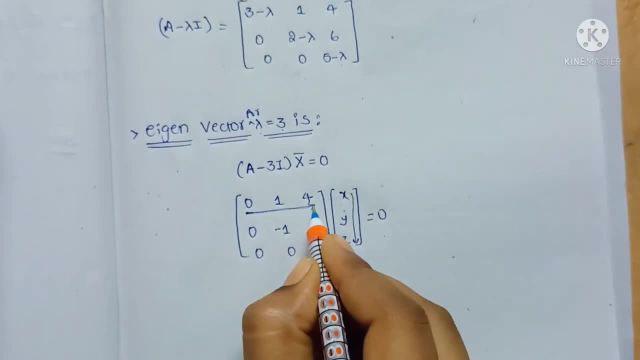 in equation form and multiply with these row into this column, we get equation from 0 into x, 0 and 1 into y. y plus 4 into z, 4 z, which is equal to 0, and similarly minus 1 into y, minus y plus 6 into z, 6 z, equal to 0. here 2 into z, 2 z, which is. 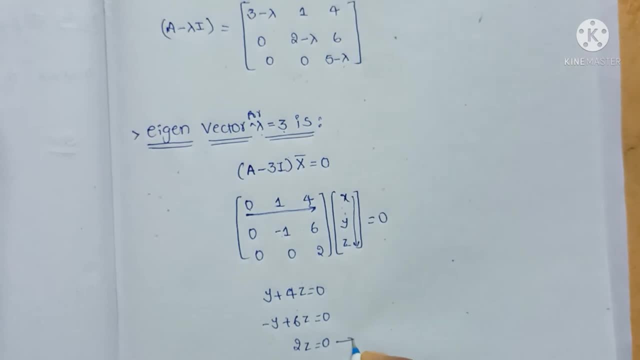 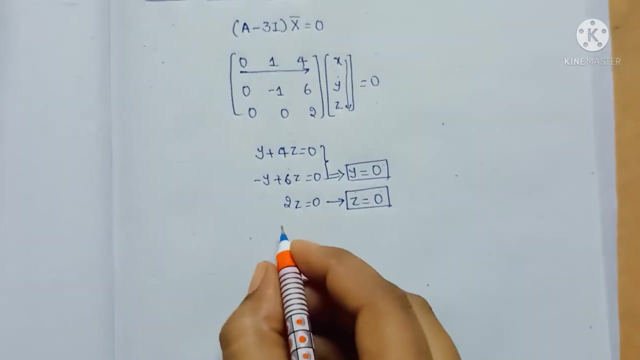 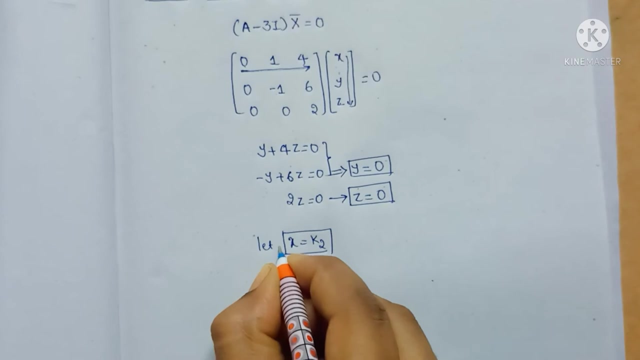 equal to 0. okay, from this equation we conclude: z is equal to 0. if you substitute z equal to 2, in case of z we get 1 minus 2 where the z is tau. so that's why this set vector is not given here a triple vector vector. so this x letter is equal to: 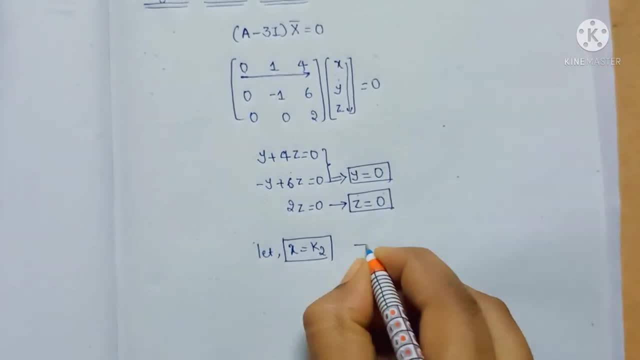 z. so this vector is the vector, which implies that this vector of x is equal toBy z, namely equal to z. the vertical enumeration is also. sisters will be extracted to this particular function in this particular Ä. the section of the vector as shown here is the initial. 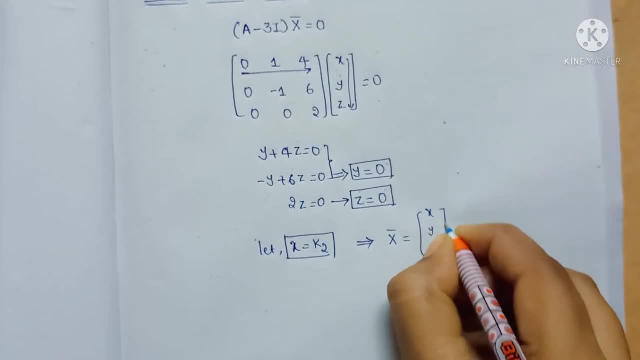 lights. first of allüzik, the factorial value in this form, and that is Psalmatics, among any porta2 values, this y is equal to y to be equal to 0. why 2? let's take all�, все corona and some немного. 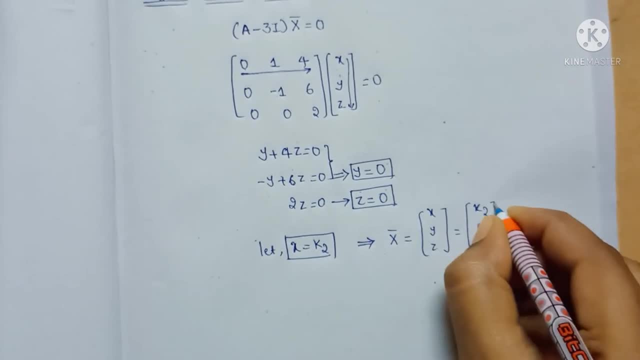 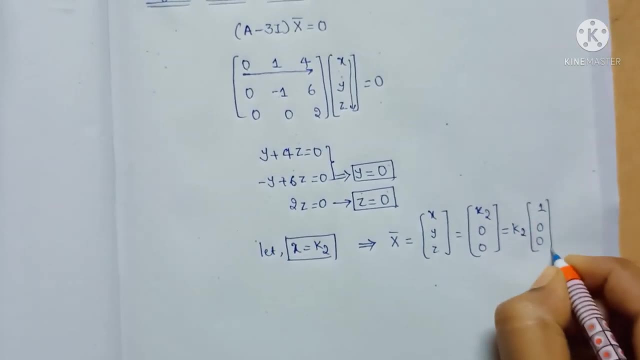 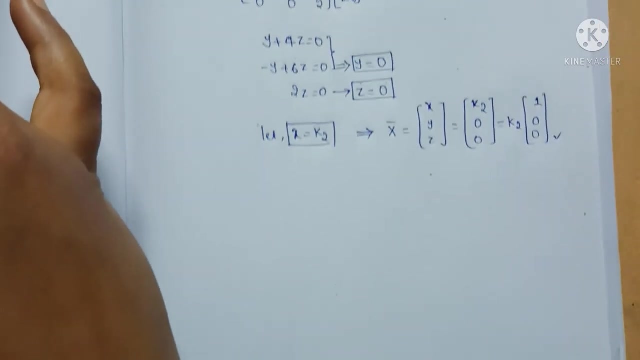 k2 and y equal to 0, z equal to 0 and by common k2 into outside the matrix, then we get 1 0, 0. this is the eigenvector for the lambda equal to 3. okay, and now we have. we have to find: 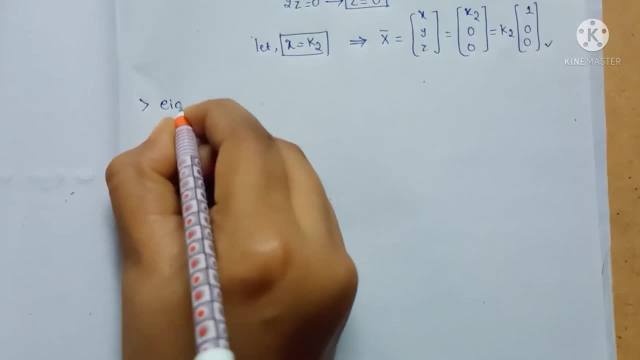 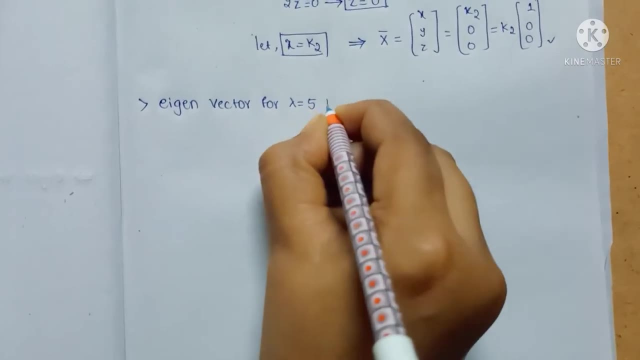 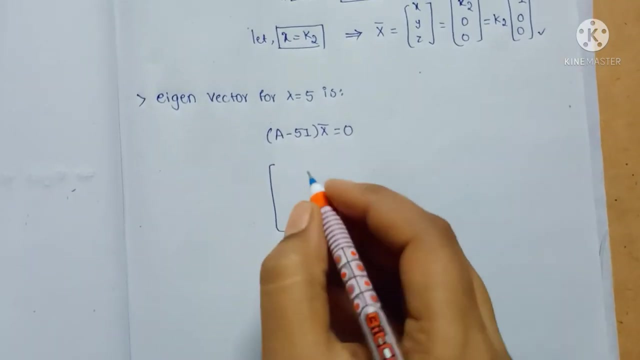 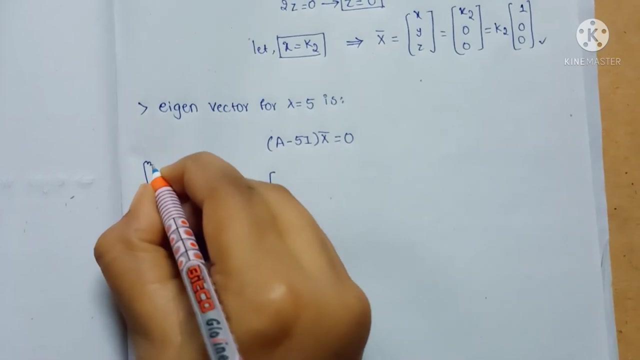 one more eigenvector: okay. eigenvector for. lambda equal to 5 is okay. eigenvector for. and now i am getting here: 3 minus 5. okay, sorry, here i am writing a minus lambda, a matrix: 3 minus lambda. 1, 4, 0, 2 minus lambda. within a matrix. we have v-r and 2 minus lambda, so that's the eigenvector for lambda. we have to use a: 1, 0, 2, 0. if you give me any, a minus lambda, i matrix b minus lambda, i 1, 0, 0. if you give me any, an matrix, ok, and now i amici t1, ,1, 0. and now i have to use ad features. 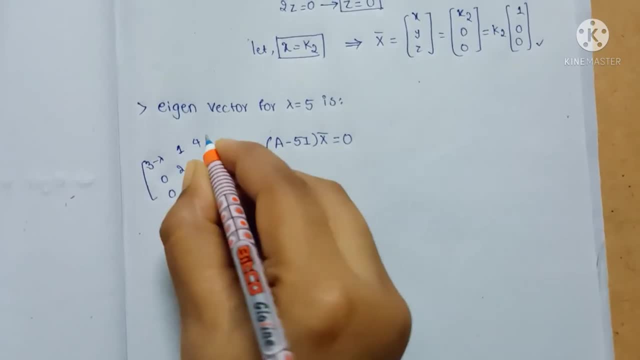 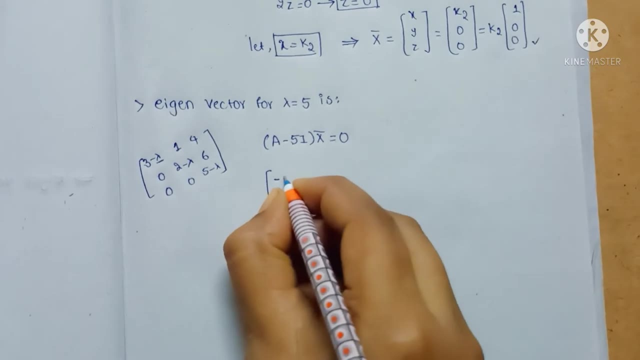 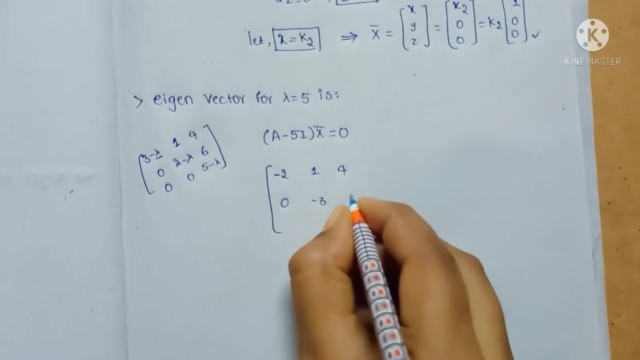 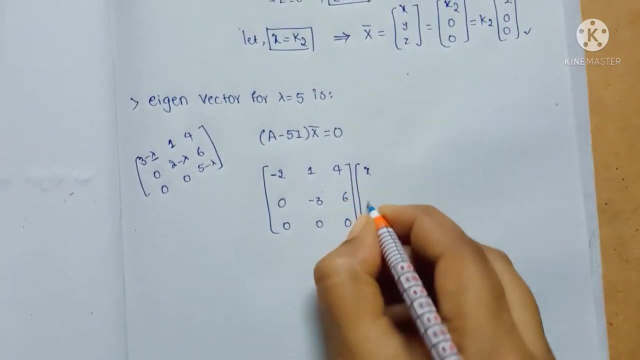 6, 0, 0, 5 minus lambda. okay, here in place of lambda we are substituting 5, 3 minus 5. we get minus 2. and 1, 4, 0, 2 minus 5 get minus 3, 6, 0, 0, 5 minus 5, 0. and where x bar is the x y z vector, which is: 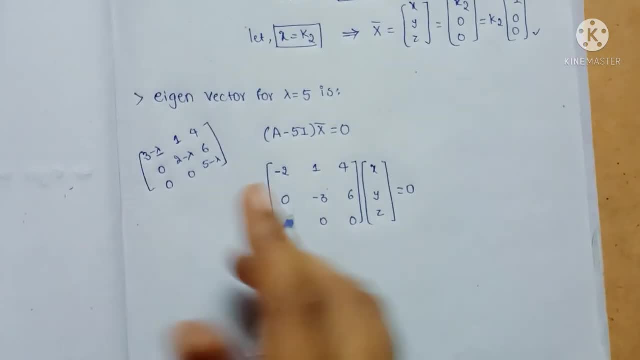 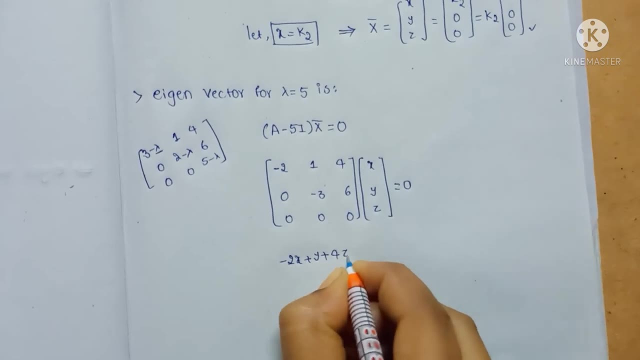 equal to 0, and now we are writing these in equation form: is minus 2 into x, minus 2, x plus y plus 4 z equal to 0. and similarly for next row: minus 3 y plus 6 z equal to 0. okay, value.